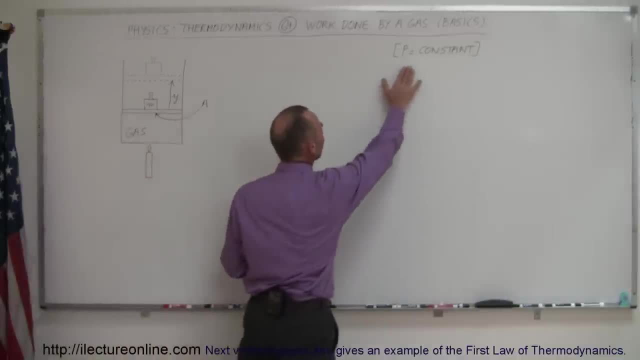 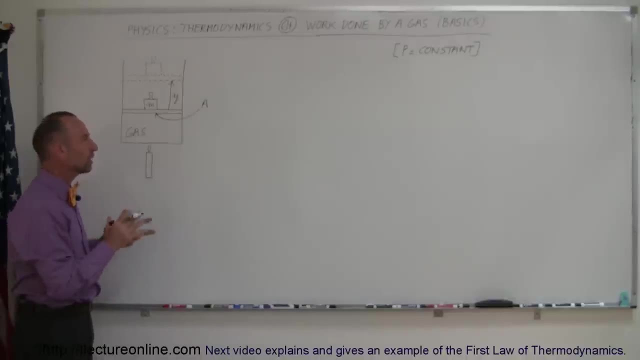 that in a simplistic case- and the simplistic cases where in this case we're going to leave the pressure constant, so the state variables of course are pressure, volume and temperature. so in this case we're only going to deal with volume and temperature. and here's our example. let's say we 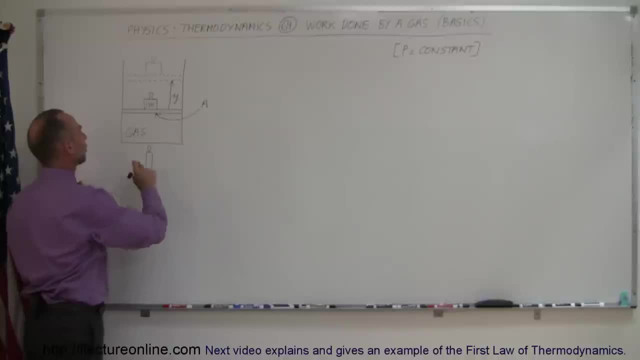 have a piston. we put a weight on the piston so that it's pushing down against the the piston here. and we're going to put a weight on the piston so that it's pushing down against the the piston here. and and when we add heat to the gas, the gas absorbs that energy, use that energy to do work and pushes. 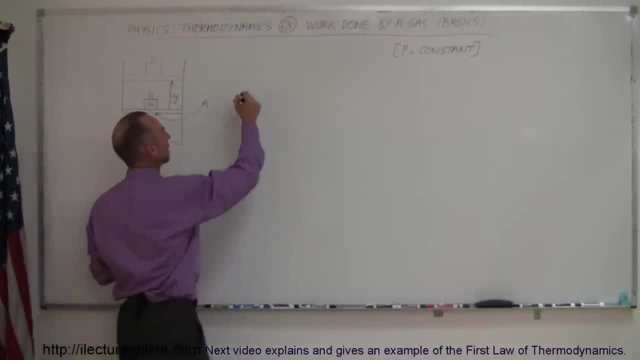 the piston up to a new location right there, so we can say that the work done is equal to force, times, distance. and, of course, what is the force that causes this piston to go up? it's the force, force caused by the pressure inside the gas, and so know, by definition, that the pressure inside 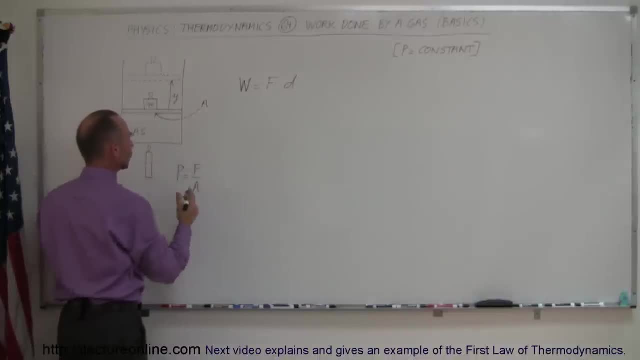 the gas is equal to force divided by the area over which the pressure occurs. and since the gas is flowing where it's moving, at the end, of course, the distance over which, of course, is basically the pressure, along with the position of force, then that goes by the distribution. 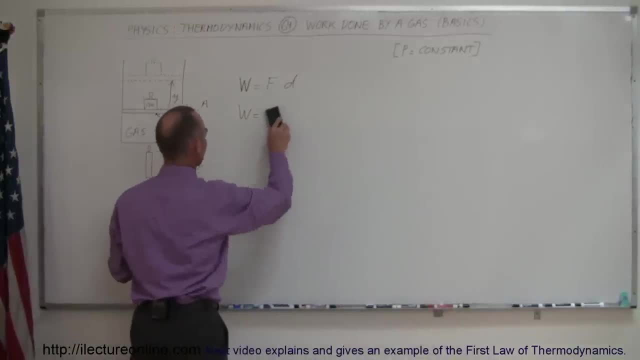 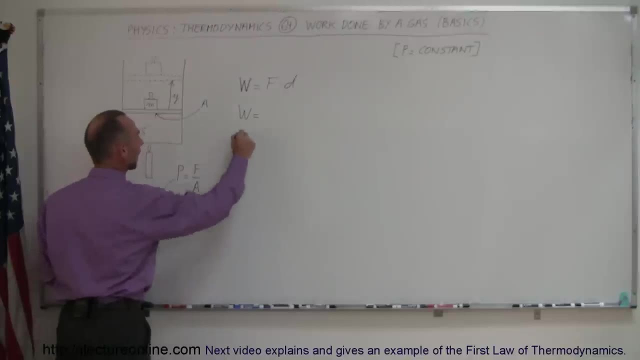 and part of the pressure that we're giving to the heat is the pressure p string share power which transactions from the equation department here to the sector. and let's start this way. so we have force equal to pressure times weight divided by go f and that by square root of force. an x cross over dels tis is equal to theopathic fifteenде shapes, and of course we have the cross section area of the piston here, which means that the work done is equal to the pressure divided by. uh, i'm sorry that's not going to be correct. uh, let's see here, because i 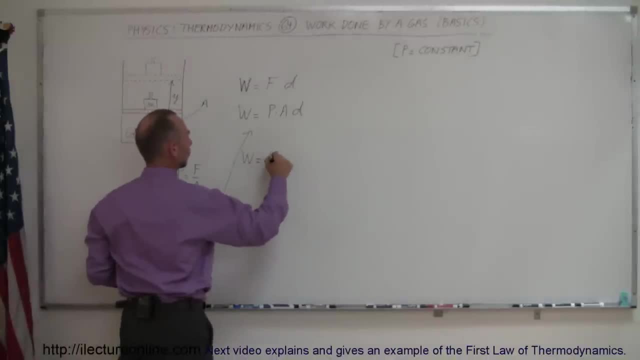 from here to there. so we can say that the work done in this case is equal to pressure times, area times the height that the piston gained and, of course, the A times the Y. this portion of the equation is equal to the change in the volume. cross-sectional area times height is the change in the volume right here. 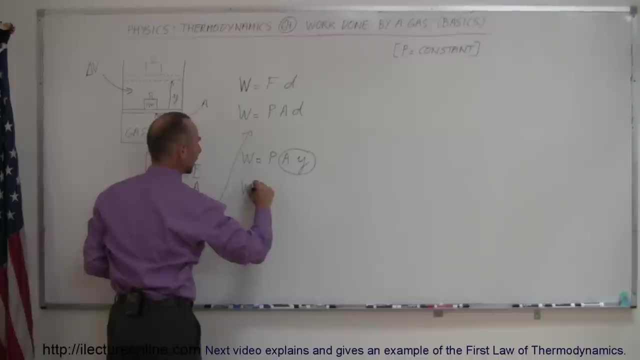 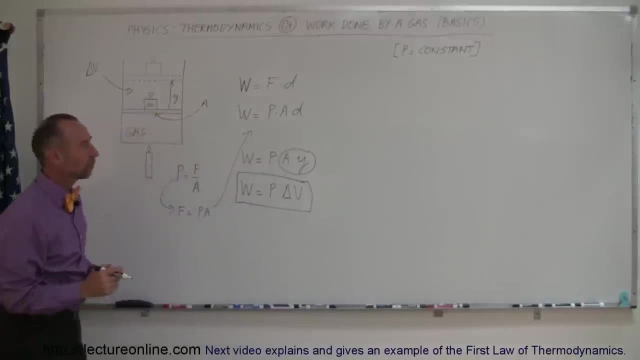 that's your Delta V, and so we can say that the work done by the gas is equal to the pressure times the change in the volume of the gas, and that is a simplistic way of looking at how work is done in the gas. it's simply the. 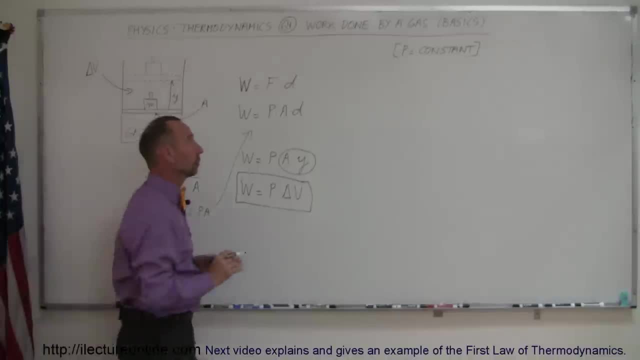 pressure of the gas times the change in the volume, taking into account that in this case the pressure is constant. so if we want to put some units on that, let's say that the cross-sectional area area is equal to, let's say, 50 square centimeters, and let's say that the pressure P is equal to: how about 1.5? 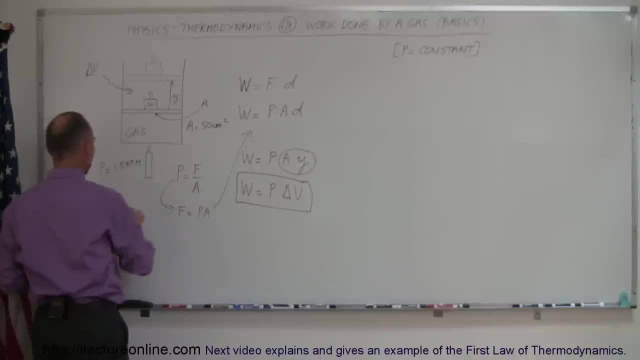 atmospheres, and let's say that the height gained Y is equal to 10 centimeters. so what is the work done in this particular case? all right, well, first of all, we're going to convert these units to standard units. atmospheres has to be converted to Pascal's or Newton's per square meter. 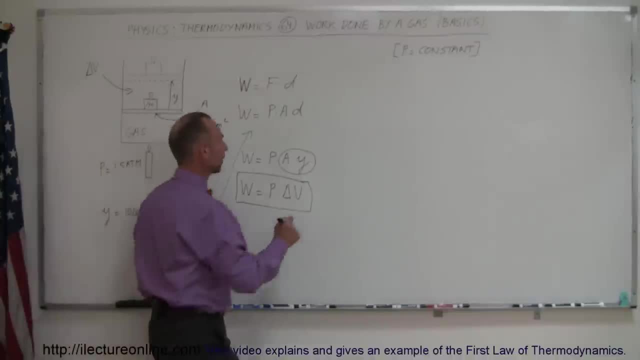 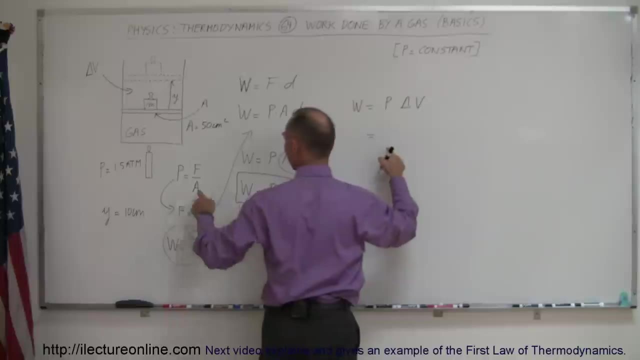 and of course centimeters will have to be converted to meters. so the work done in our case here is equal to pressure times. the change in the volume and the pressure is 1.5 atmospheres and of course that has to be converted to Pascal's. 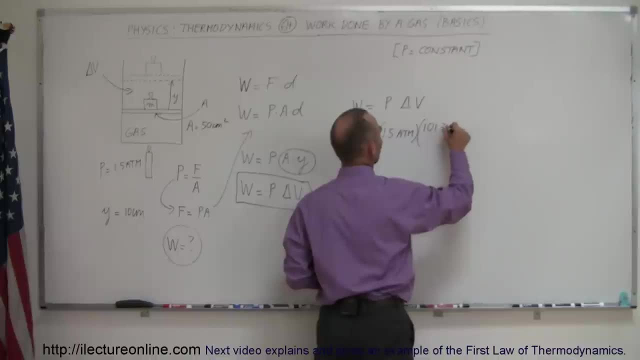 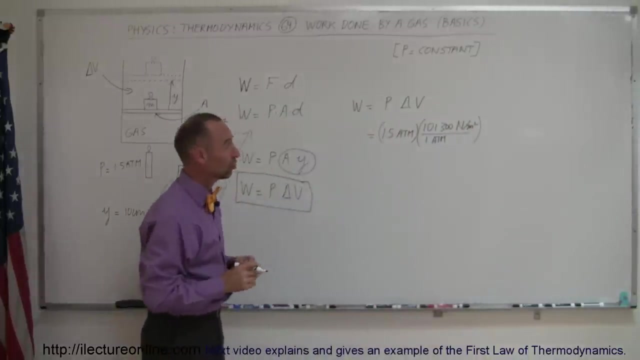 which is 101,300 Pascal's or Newton's per square meters per 1 atmosphere. so maybe I'll just go ahead and write it like that so it makes a little simpler. so that's pressure changed to Newton's per square meter and the change in 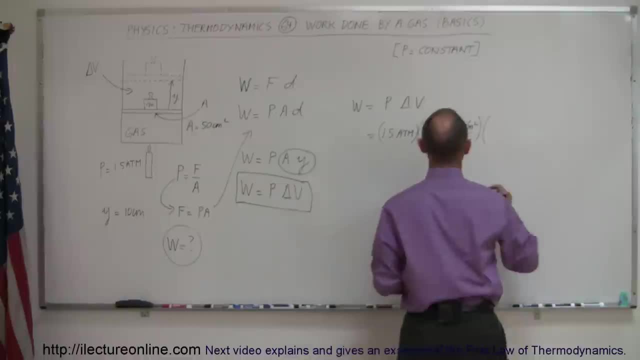 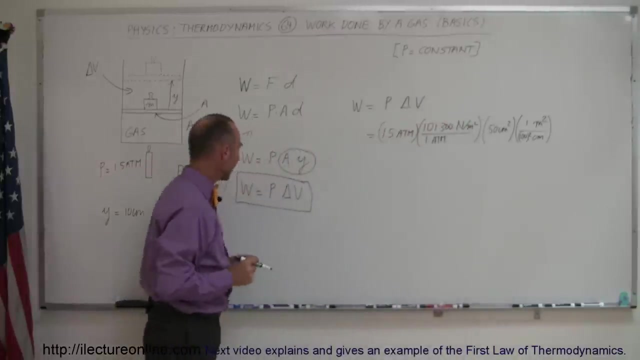 volume is going to be, in this case, the cross-sectional area. that would be 50 square centimeters, which is converted to square meters. so we need meters squared here and centimeters. one meter is a hundred centimeters and we have to square that and then finally, the height. it gained a distance of 10 centimeters. so 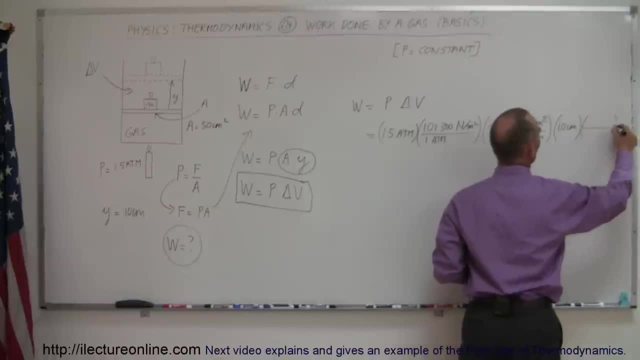 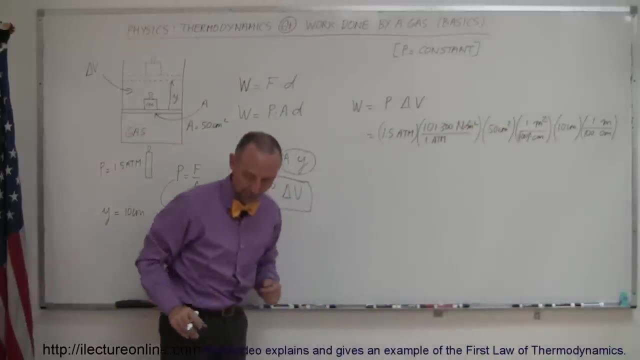 that would be 10 centimeters, and also that needs to be converted to meters. so I have meters and centimeters, and there it's: one meter is a hundred centimeters. we don't have to square that, because that's a linear unit. now, using my calculator, let's see what the work then is in this particular case. yeah, so we.